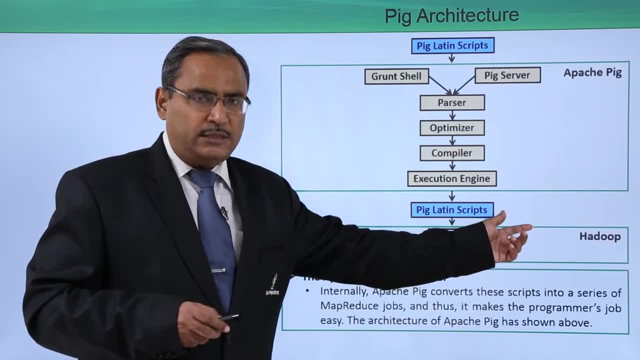 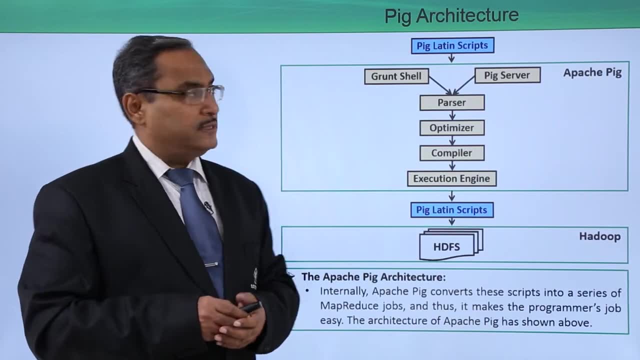 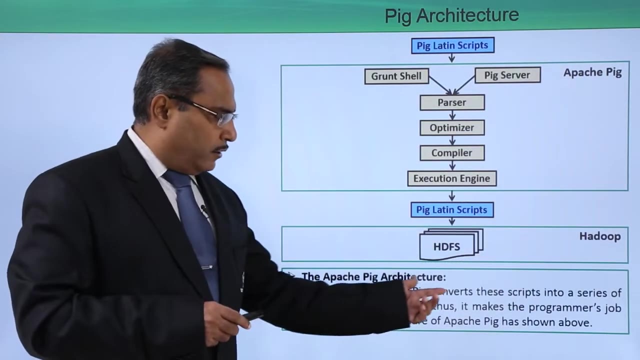 be assigned to this Hadoop, So Hadoop will be executing those tasks. those map reduce tasks. and after accessing the HDFS, that is a Hadoop distributed file system And there is a PIG architecture we have discussed using this diagram Internally. Apache PIG converts this. 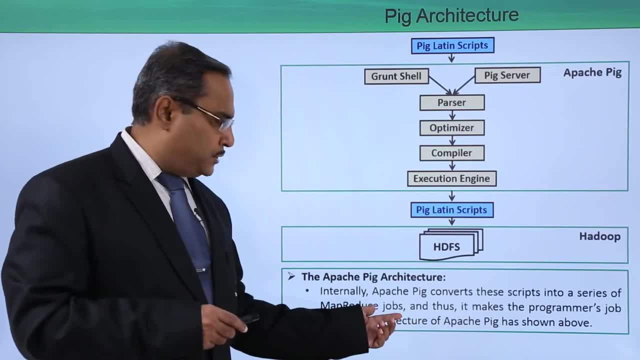 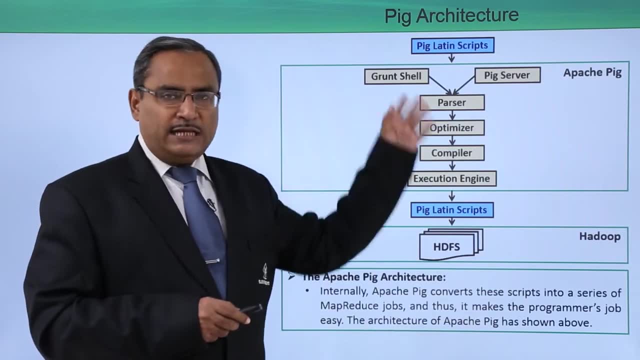 scripts into a series of map-reduced jobs, and thus it makes the programmers' job easy. And the architecture of the Apache PIG has been shown above. So this is the architecture, and using this architecture, phasewise, the operation is successful in this way. So 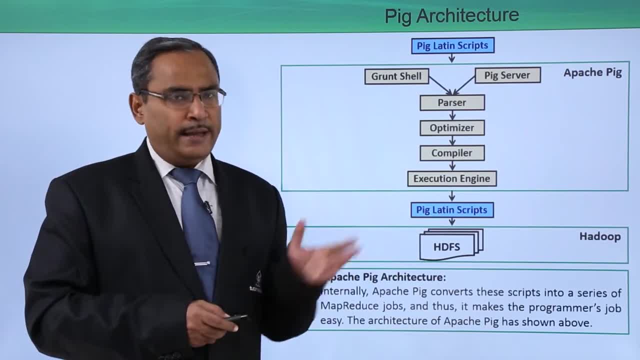 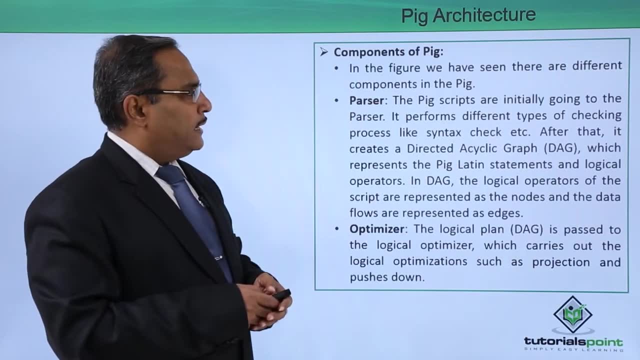 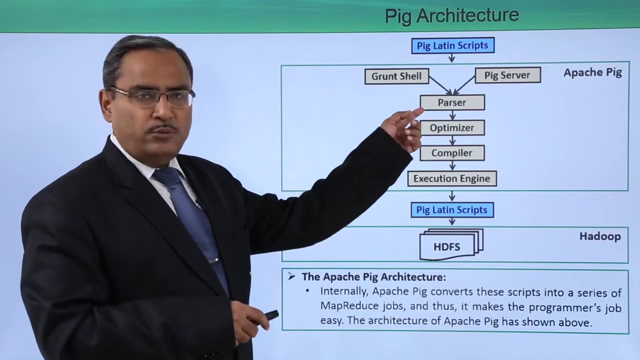 operations have to be carried out. so let us go for more detailing about this phase: wise operations. so in the figure we have seen there are different components in the peak architecture. so the first one is a parser. you can easily follow that, the first one. we are considering this one as parser. 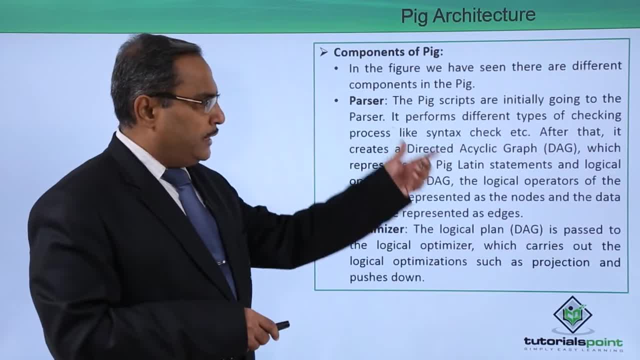 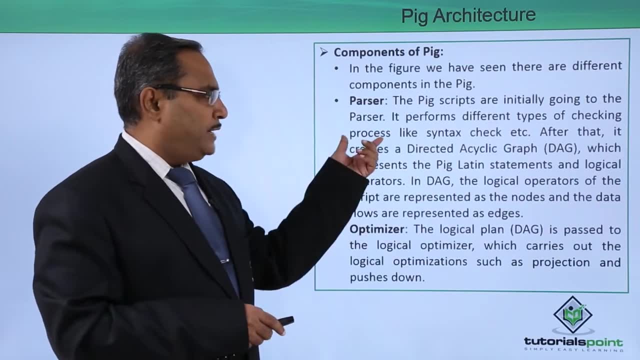 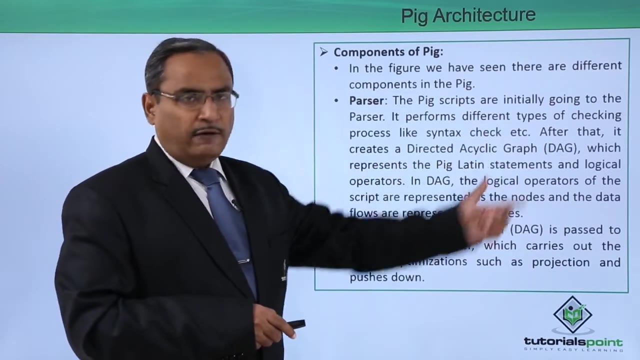 so the peak scripts are in, initially going to the parser. you can find that peak scripts are going to the parser at first and it performs different types of checking process, like the syntax check etc. and after that it creates a directed acyclic graph. there is a dag, and which? 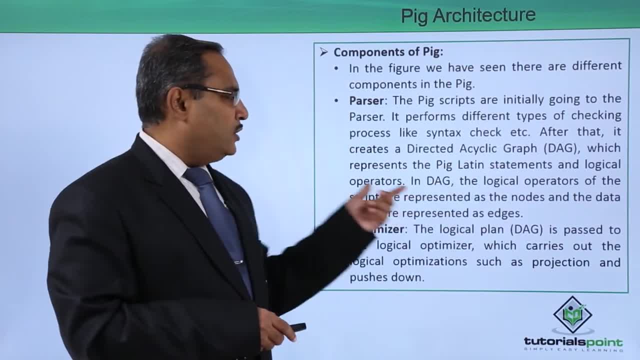 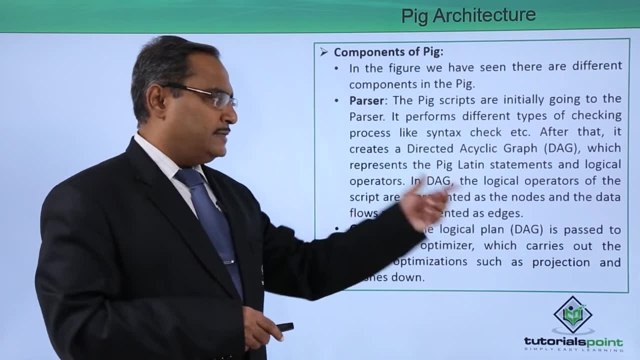 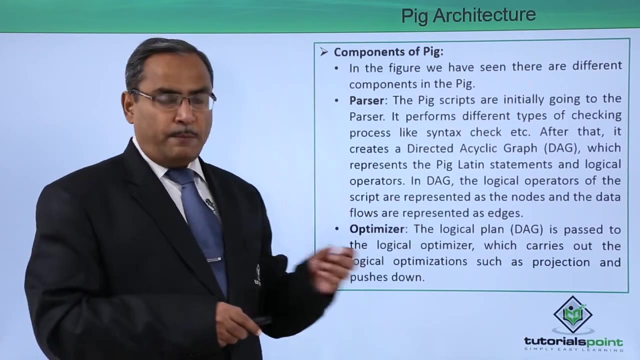 represents the pig latin statements and the logical operators. and in dag the logical operators of the script are represented as the nodes and the data flows are represented as the edges. so these operations will be denoted by the nodes, because directed acyclic graph graph means we know that it will be. 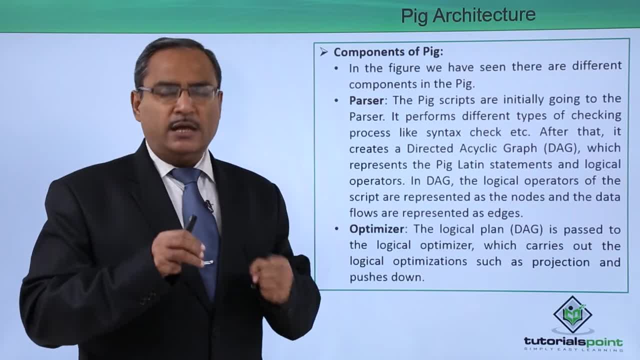 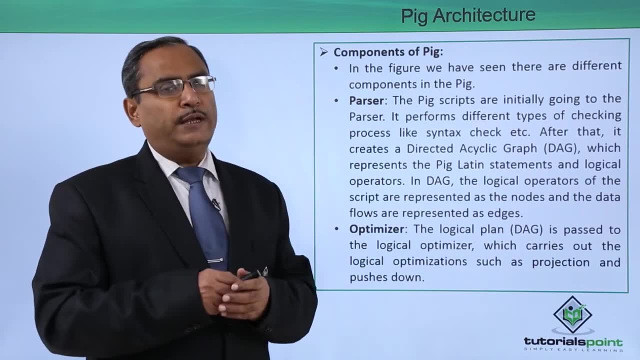 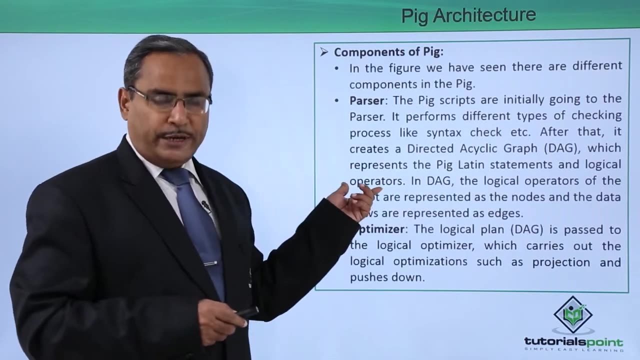 consisting of multiple number of nodes and the edges. these nodes will be nothing but the operations to be carried out by the operators and this edges will be denoting the flow of data. so the, which represents the pig letting statements and logical operators. so dag will be representing 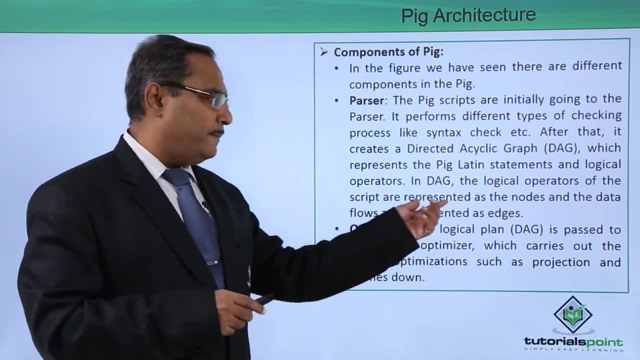 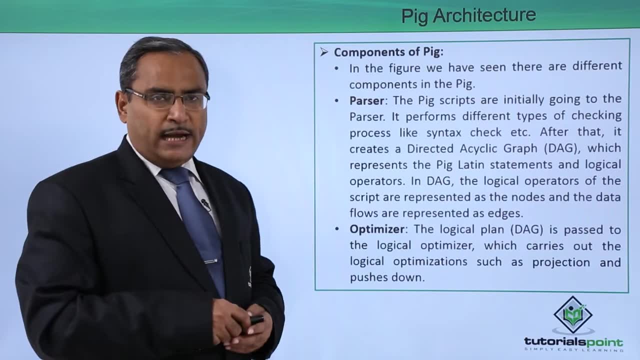 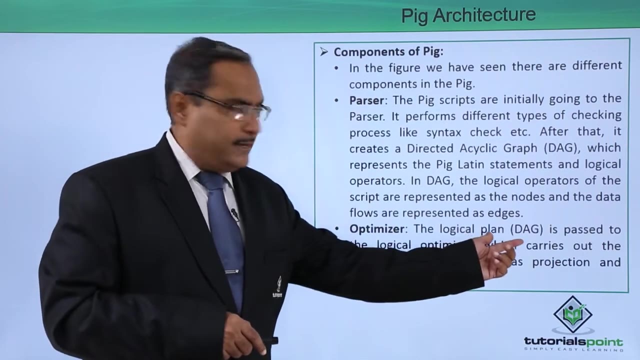 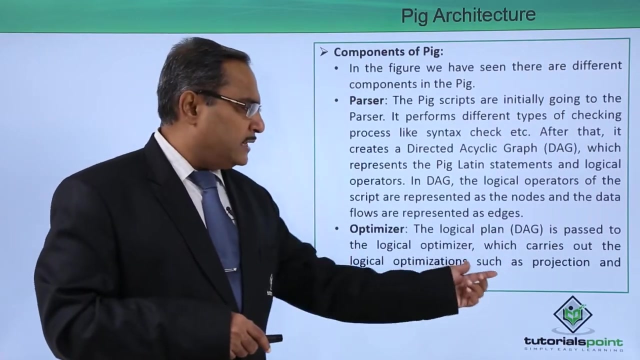 this: in dag, the logical operators of the script are represented as a node and the data flows are represented as edges. next one: we had our optimizer. so after parser, we are having optimizer. so optimizer- the logical plan that is a dag- is passed to the logical optimizer, which carries out logical optimizations, such as the projections and pushes down. so this is.